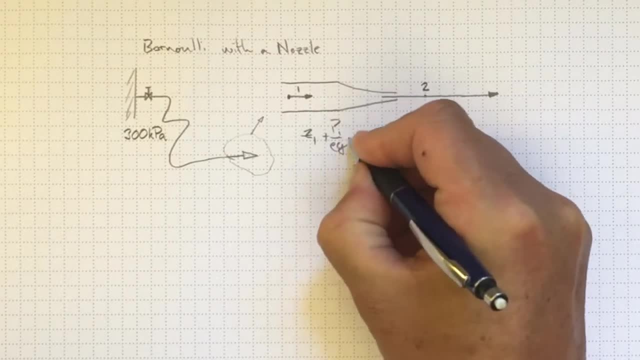 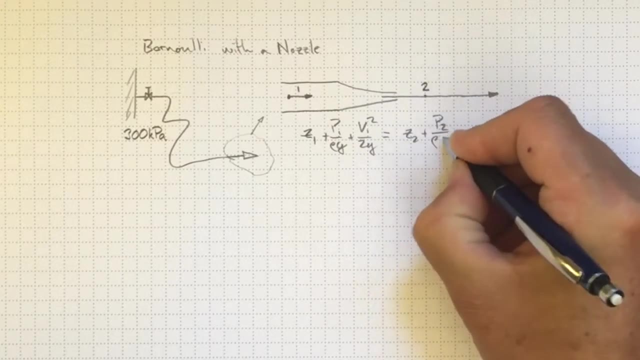 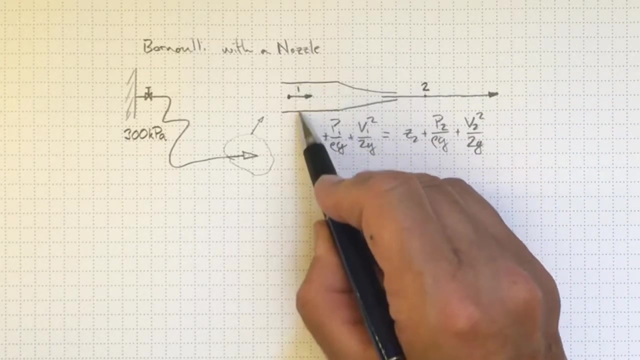 z1 plus p1 over rho g plus v1 squared over 2g must be equal to z2 plus p2 over rho g plus v2 squared over 2g. Now if we assume that this hose is really large compared to the outlet, 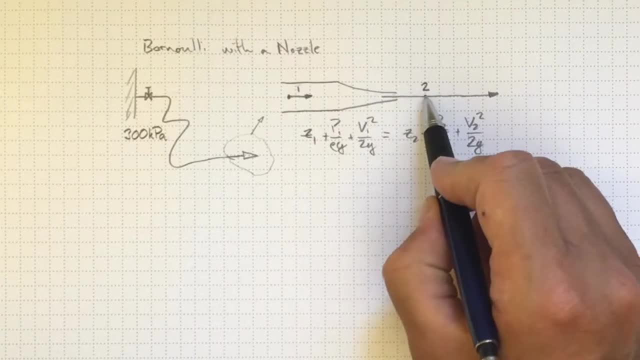 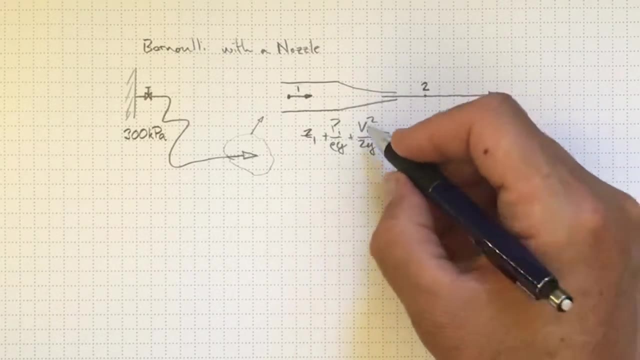 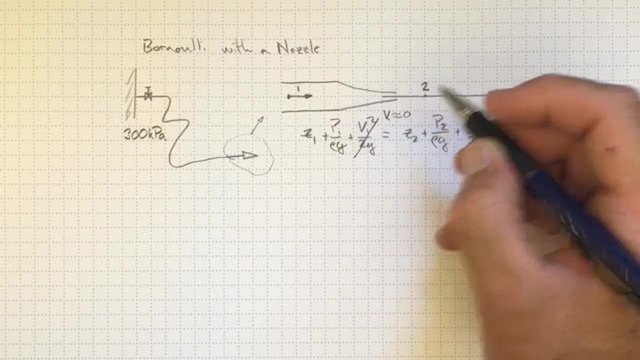 diameter of the nozzle, we can say that v1 is going to be much smaller than v2, or at least certainly v1 squared is going to be much smaller than v2.. So we'll start off by saying that v1 is approximately equal to zero. It isn't actually, but it's close. Likewise, if this nozzle is: 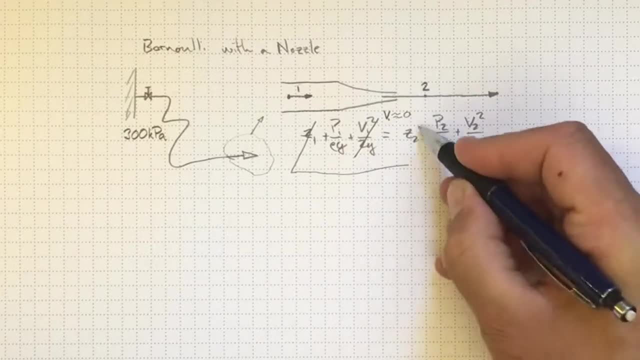 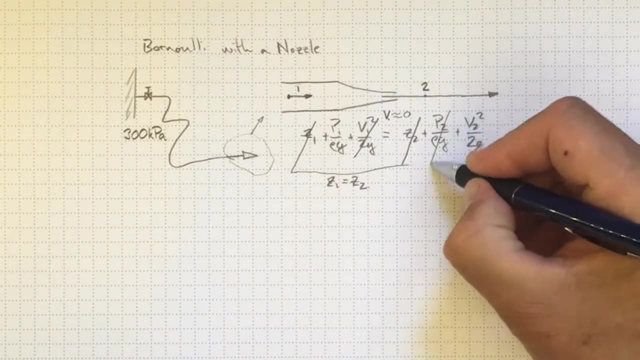 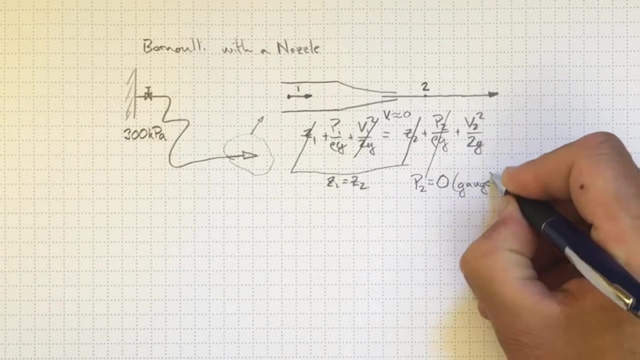 horizontal. the elevation doesn't change between location 1 and location 2.. So whatever z1 is, z2 is the same. p2?? p2 is atmospheric, It's equal to zero. That's a gauge pressure relative to atmospheric. so we better make sure p1 is the gauge pressure. And when we talk about municipal, 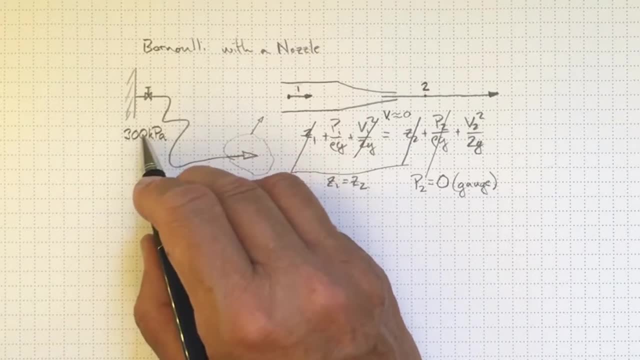 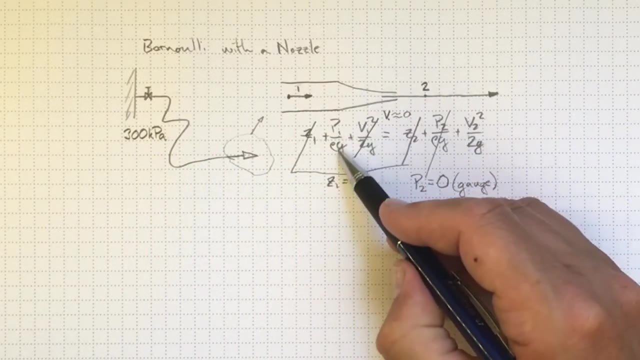 water pressure supply. we're always talking about how much higher pressure than atmospheric pressure anyway. So this is a gauge pressure. So now we've got just p1 over rho g and v2 squared over 2g. The higher the pressure, the higher the 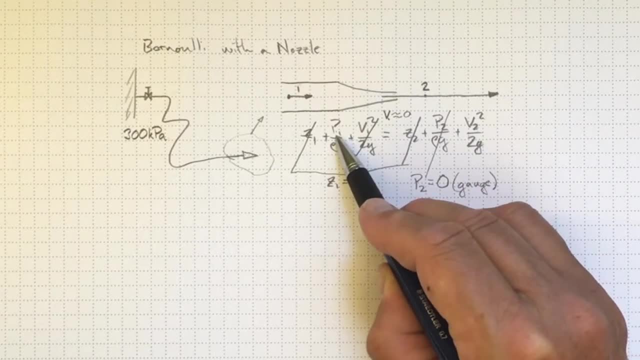 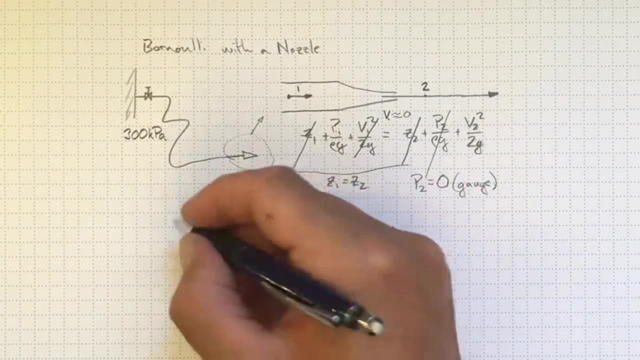 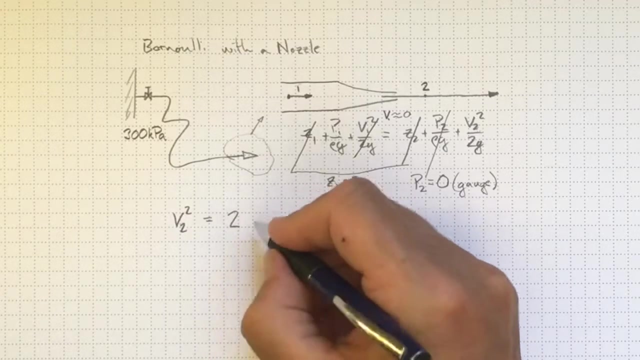 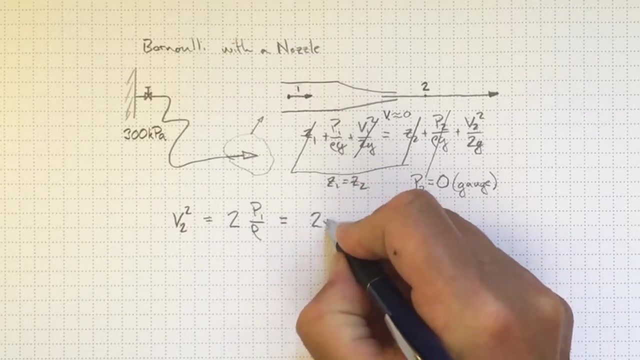 velocity squared is going to be as we convert potential energy of pressure into kinetic energy of velocity through this nozzle, So rearranging, we'll get v2 squared equal to 2 times p1 over rho, Because the g's will cancel out. That'll be 2 times 300 kilopascals, That's 300 times 10. to the third. 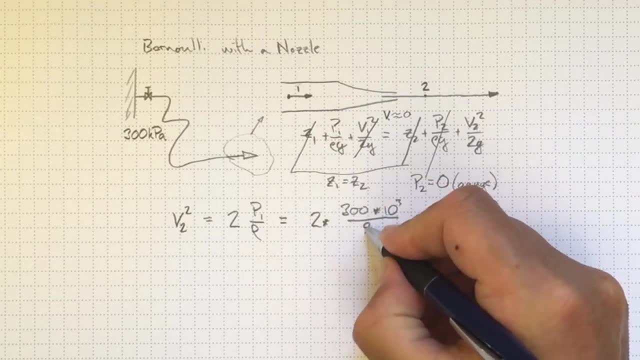 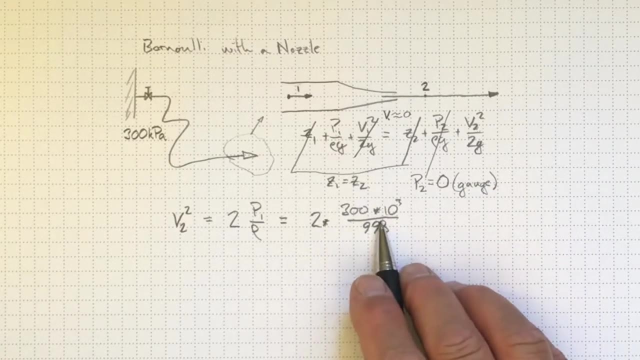 divided by density, Density of water at 20 degrees C is about 998 kilograms per cubic meter. So if we punch these in, the units are all consistent- We'll wind up with v2 after we take the square root, equal to 24.5.. 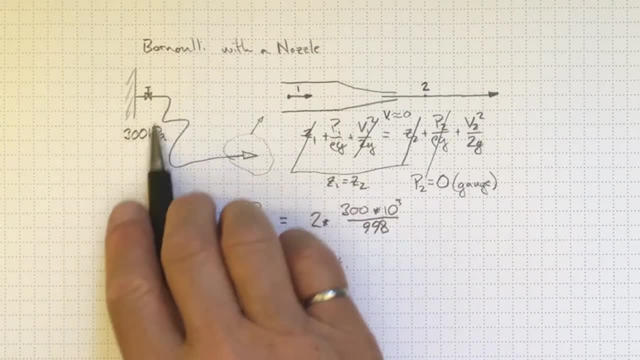 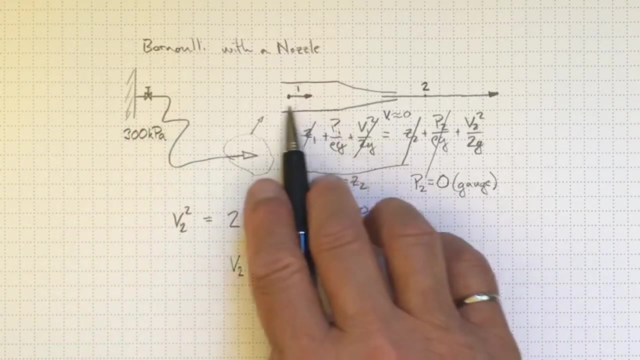 meters per second. So we looked at a typical garden hose at a supply pressure of around 300 kilopascals, That's around 45 psi, about three atmospheres above atmospheric pressure, Not atypical for a municipal water supply. In this hose it was going very slowly, but the pressure